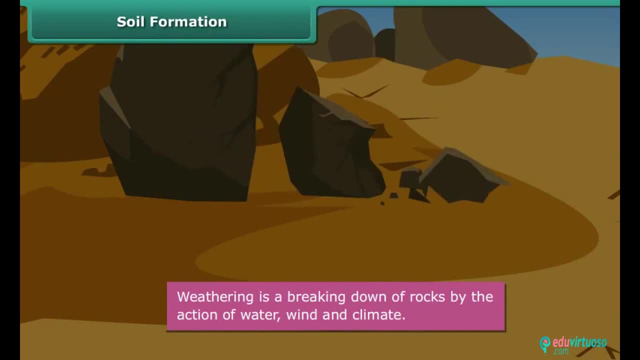 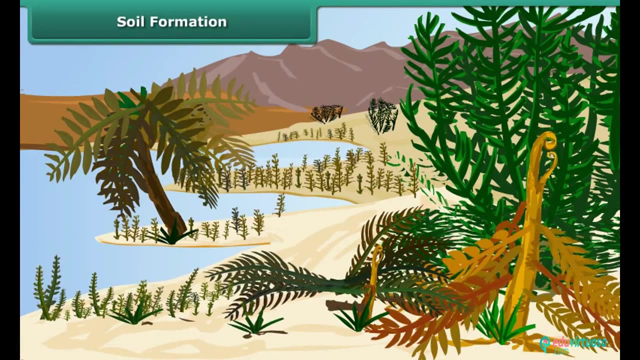 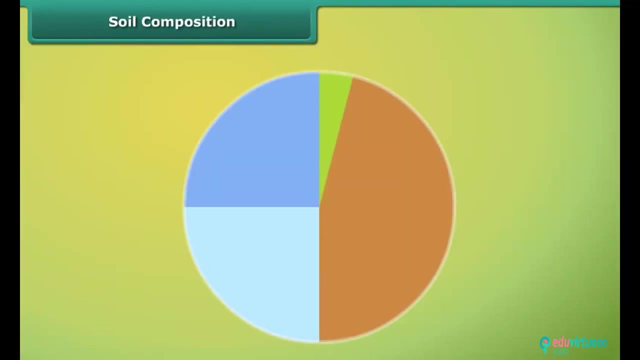 and finally to soil, by the action of wind, water and climate in a process called weathering. also, decaying of dead plants and remains of animals made the soil thick and rich and eventually it became support for life. soil composition: soil is a mixture of water, air, parent material and organic matter. over time, these four components combine together to form healthy. 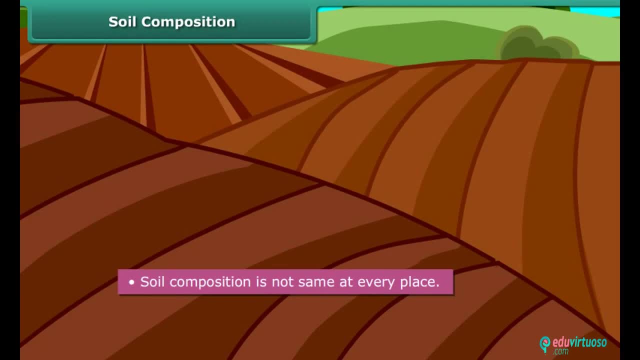 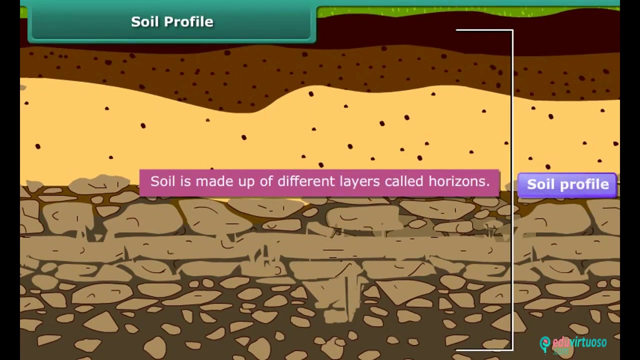 fertile soil. don't think that soil composition is same at every place. it depends on the rock from which it has been formed and the type of vegetation that grows on it. soil profile- soil- is made up of different layers called horizons. each horizon has its own characteristics. 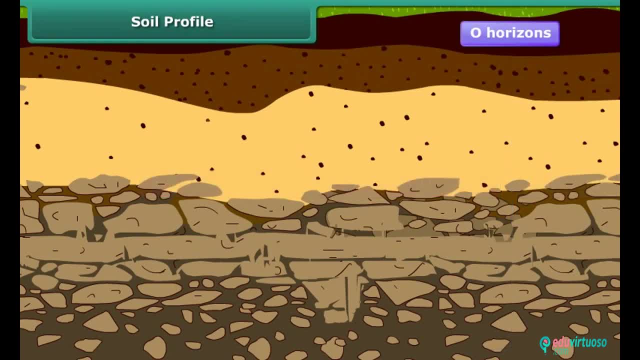 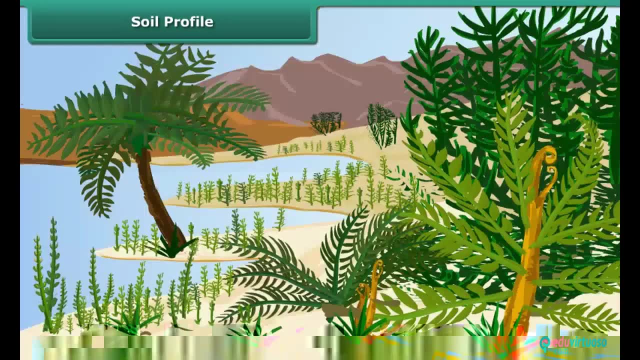 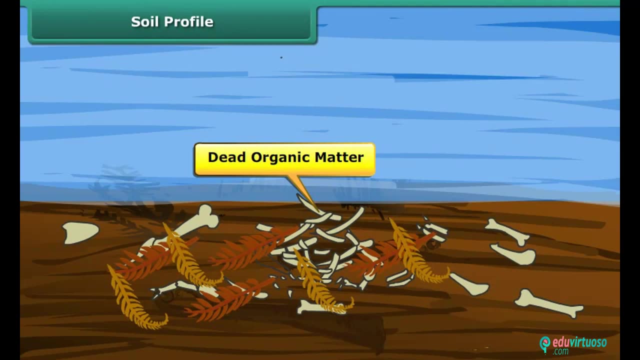 soil basically has five horizons, namely o, a, b, c and bedrock. the first layer is called the o horizon. this layer contains dead organic matter that lies on the surface. this mostly consists of fallen leaves and decaying animals. second layer is the a horizon. this is 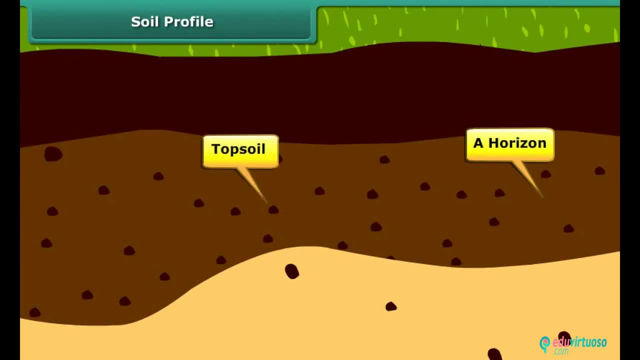 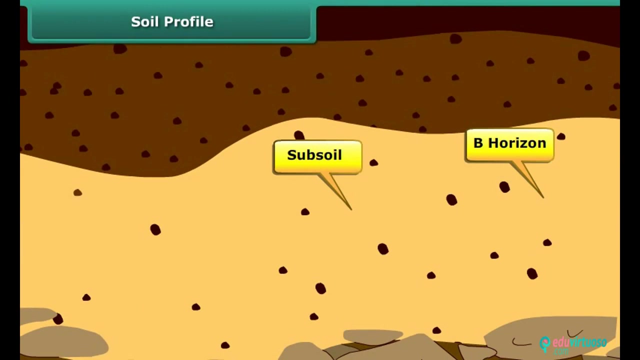 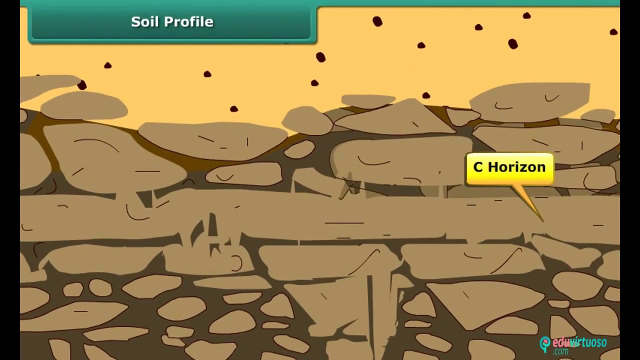 commonly known as topsoil. this layer has high concentration of organic material called humus. many living organisms live in the topsoil. third layer is the b horizon. it is commonly known as subsoil. this layer contains more minerals but less humus. fourth layer is the sea horizon. this 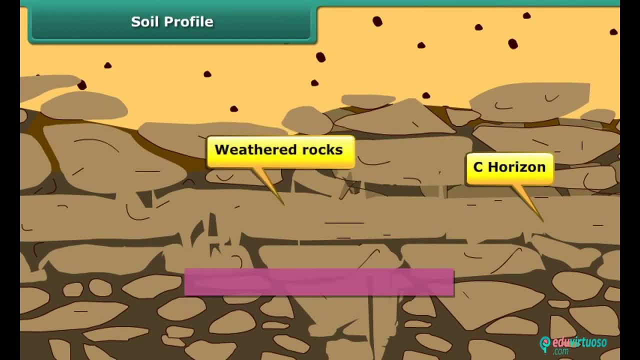 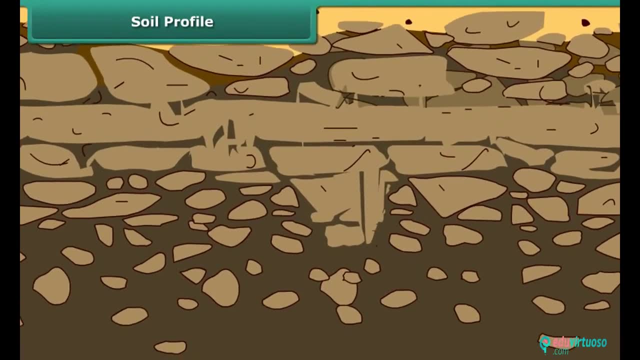 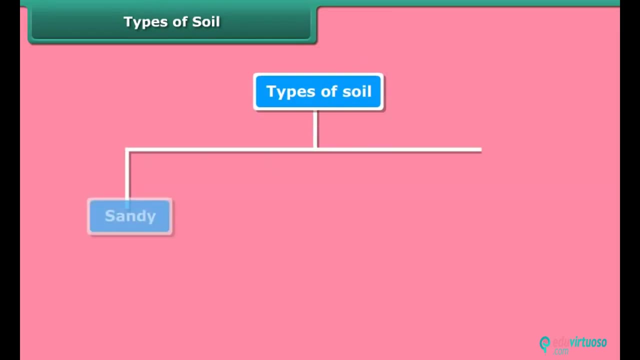 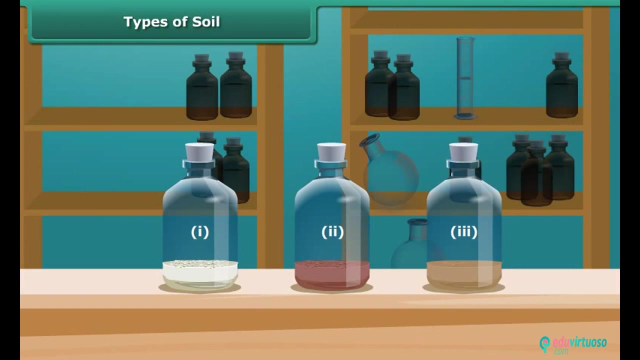 layer is rocky and made up of weathered rocks. nutrients concentration is low in this layer. the final layer is made of solid rocks and commonly known as bedrock soil. here are three types of soil. there are basically three types of soil: sandy, clay and loamy. let's take three samples of a soil and examine them one by one. we can see the first sample. 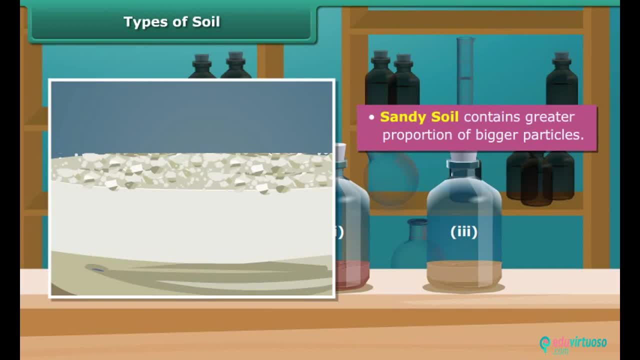 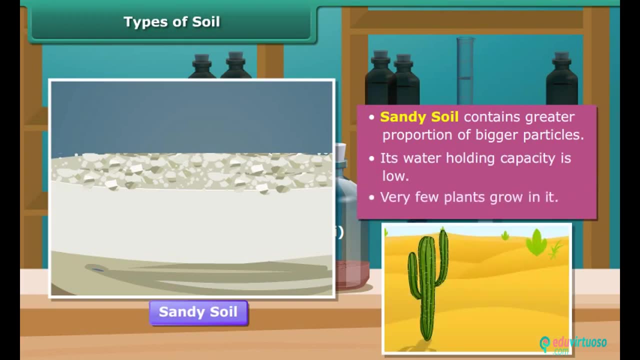 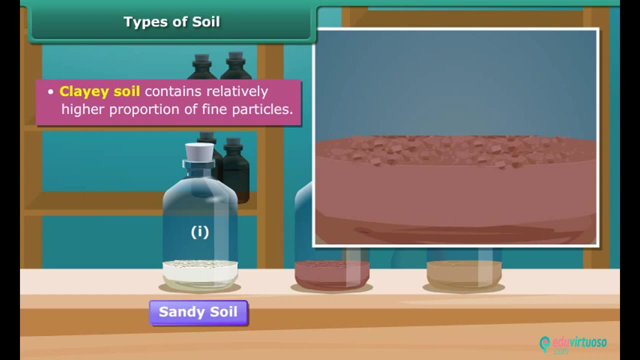 contains greater portion of bigger particles, so this is a sandy soil. its water holding capacity is low. therefore very few plants grow in it. let's observe second sample closely. it contains relatively higher proportion of the fine particles, so it is a clay soil. it is very sticky and has no spaces between the particles to hold air. therefore plants cannot grow properly in. 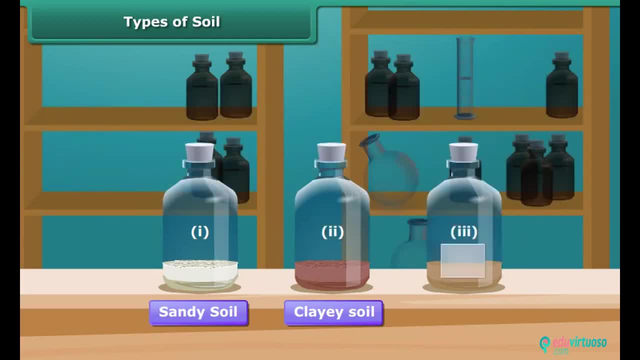 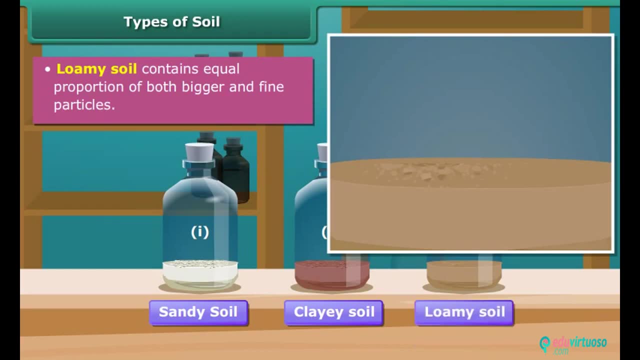 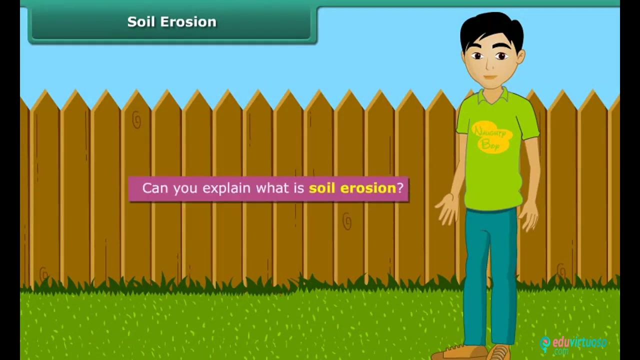 it now. let's observe third sample closely. it contains equal proportion of both bigger and fine particles, so it is a loamy soil among all the three soils, loamy soil has humus in it, which makes it fertile. also, it can hold both water and air. therefore plants grow very well in loamy soil. soil erosion: can you explain what is soil erosion? 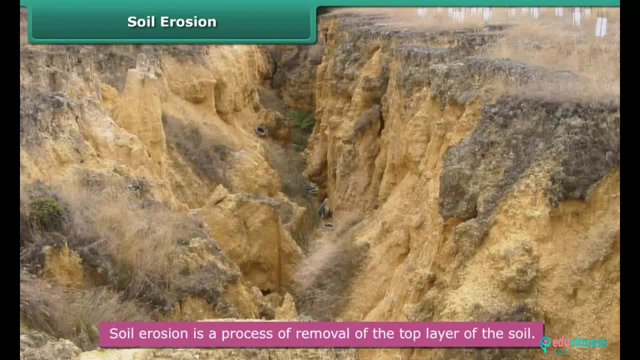 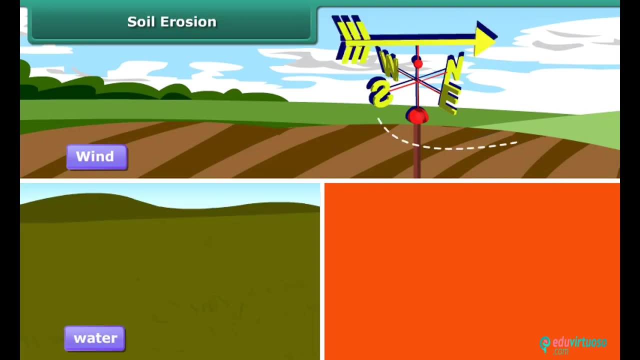 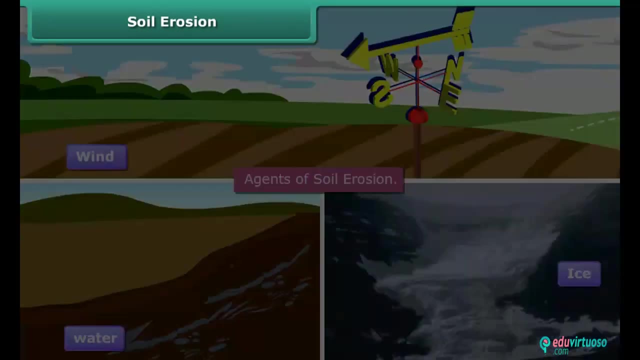 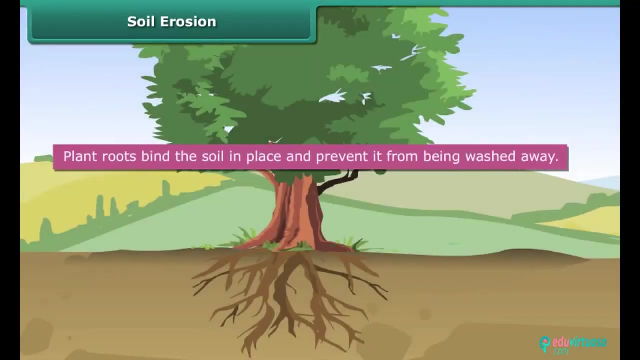 well, soil erosion is a process of removal of the top layer of the soil. but what causes soil erosion? basically, it is caused by the action of wind, water and ice. these are the agents of soil erosion. apart from natural agents, human activities like cutting down the trees also causes soil erosion. but how plant roots bind the soil in place and prevent it from being washed? 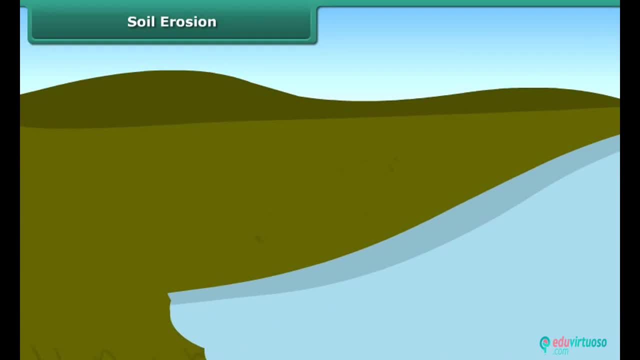 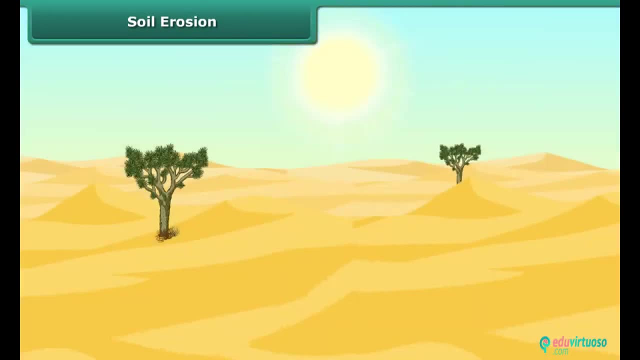 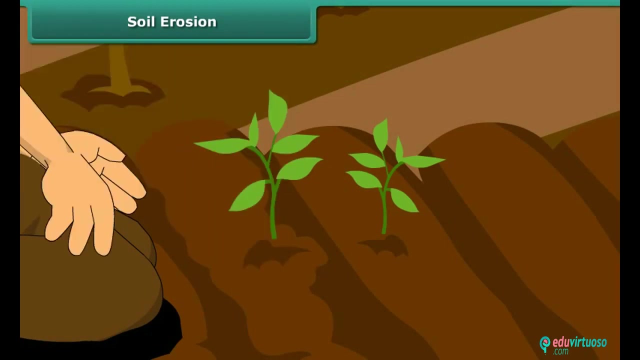 away. so if there will be no trees, floods will occur, which will leech the soil nutrients and eventually the land will become barren, which cannot be used for vegetation. therefore, more trees should be planted in order to prevent soil erosion. self-assessment: let us check what have you? 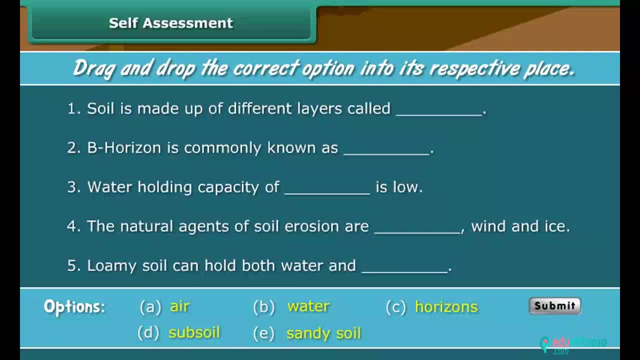 learned so far. drop your questions in the comment section and subscribe to our channel for more videos from us, and thank you very much for watching this video. hope you enjoy listening to it and till the next one, take care of yourself. Drag and drop the correct option into its respective place. 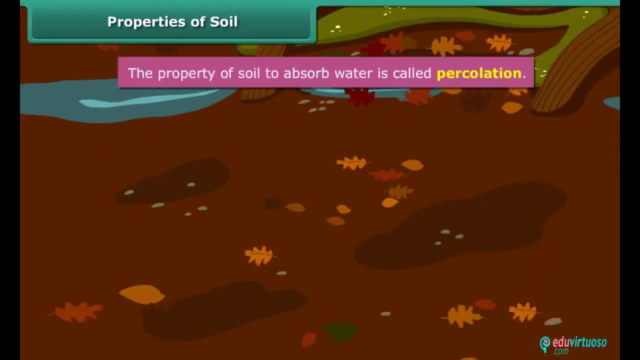 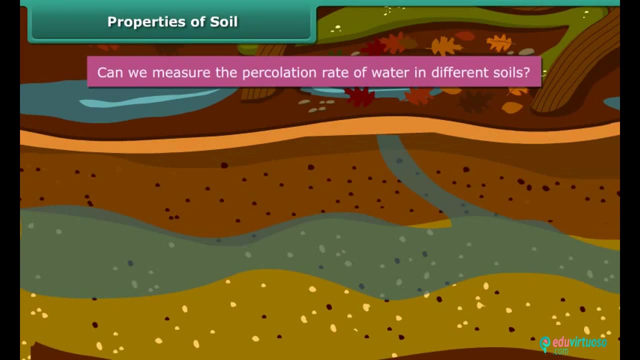 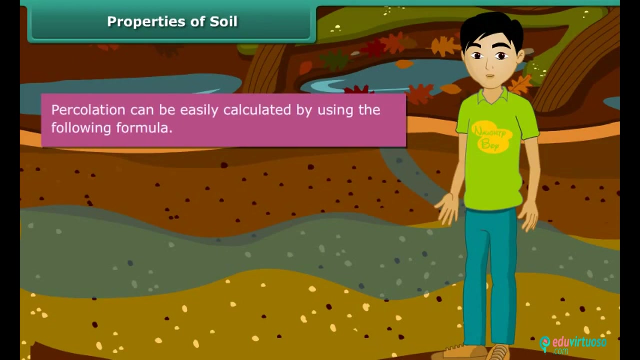 Properties of Soil. Soil has the property to absorb water. This is called percolation of water by soil. Can we measure the percolation rate of water in different soils? Yes, rate of percolation can be easily calculated by using the following formula: 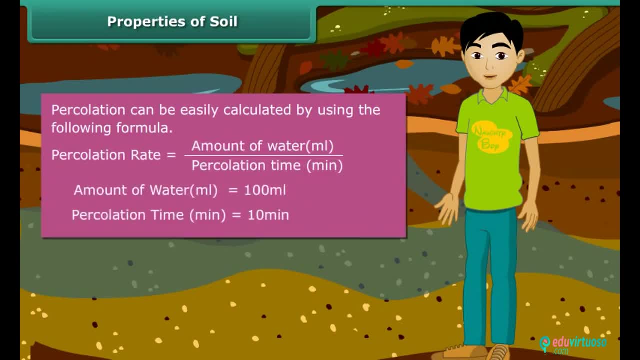 Suppose that for a certain soil sample it took 10 minutes for 100 millilitre to percolate, Then rate of percolation will be equal to 10 ml per minute. Rate of percolation is different for different soils.